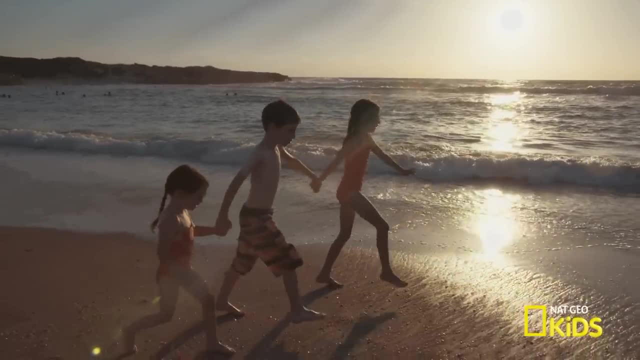 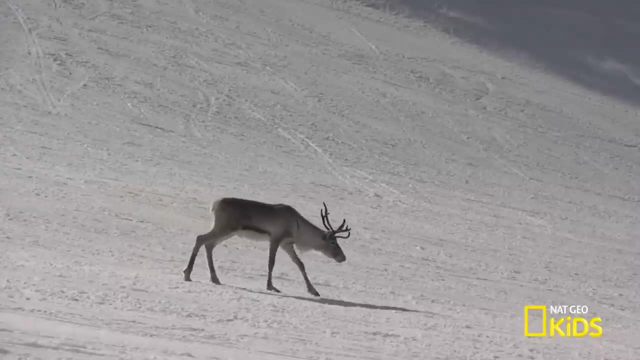 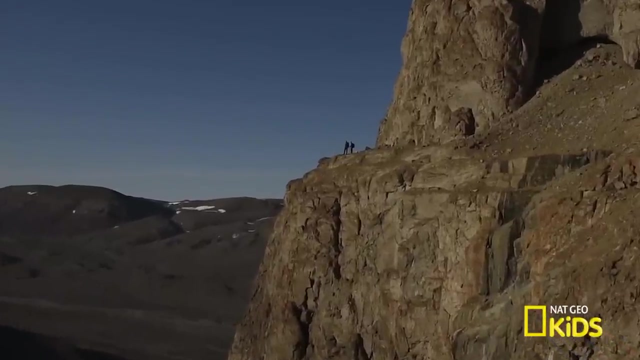 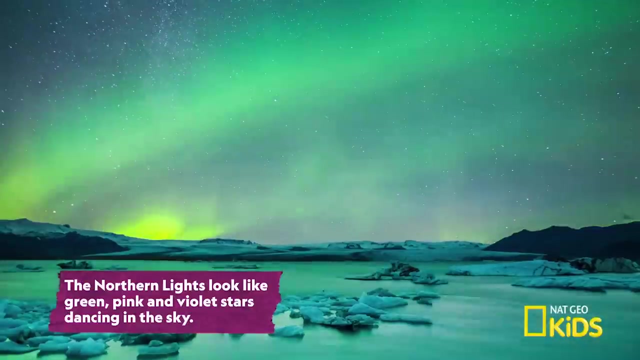 live in Europe. from the subtropical beaches of Monaco to the polar tundras of Norway, You have to brave the cold to see some of Europe's natural wonders. Iceland has one of the best views of nature's light. show the Northern Lights. If you are not. 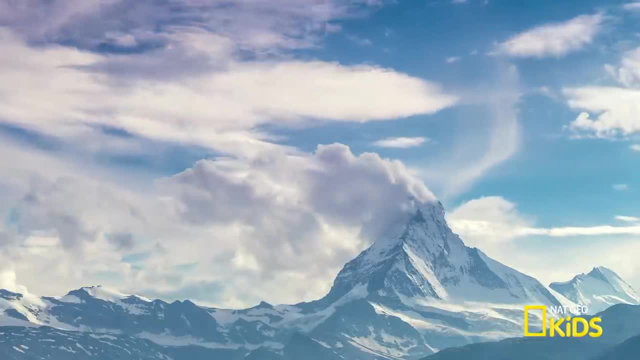 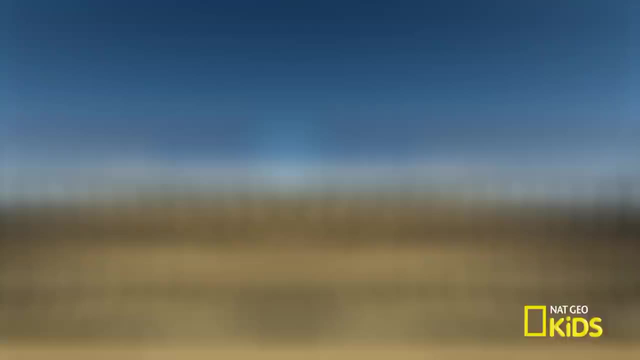 afraid of heights. head to the border of Italy and Switzerland. You can climb one of the most famous mountains in the world, the Matterhorn. It looks like a giant tooth right. Some of Europe's wonders are as beautiful as the sun. Europe's natural wonders are: 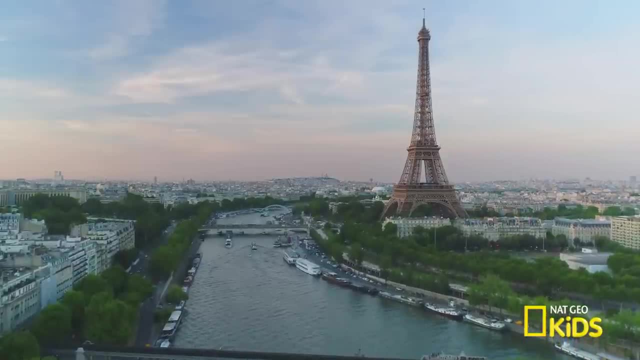 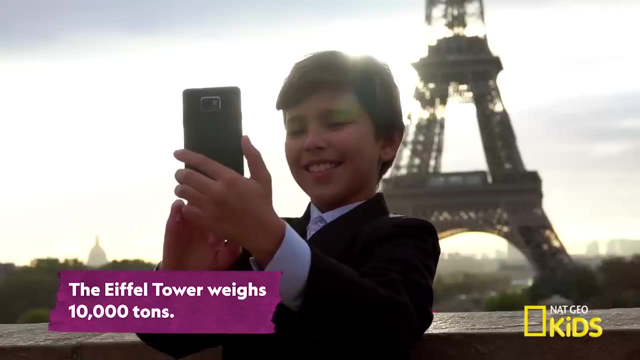 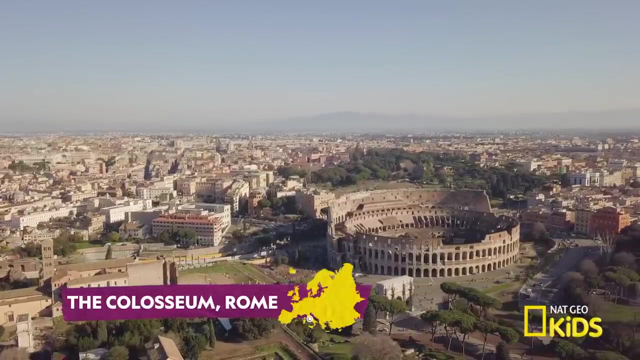 built by hand. You may have heard of a few, like the Eiffel Tower that soars above the city of Paris, France. It was once the tallest building in the world and has almost 7 million visitors every year. Or check out the Colosseum in Rome. 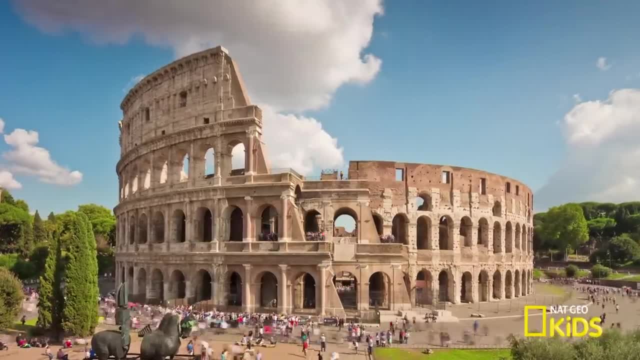 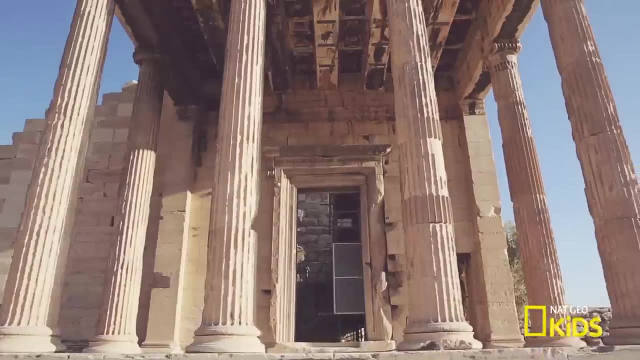 Italy. It's the biggest amphitheater in the world, made of stone and concrete and built almost 2,000 years ago. In the city of Paris, there is the most famous amphitheater in the world, the Piazza di Piazza. The Piazza di Piazza is a Roman amphitheater built in the 6th century. 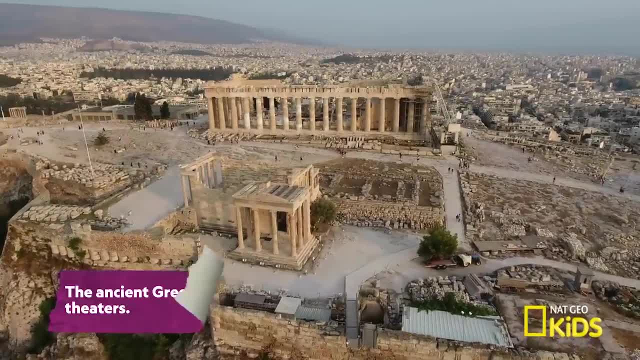 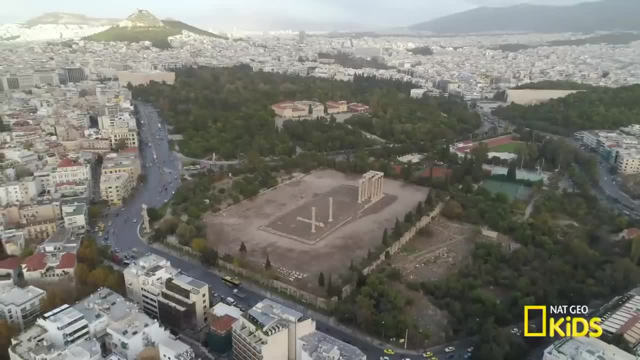 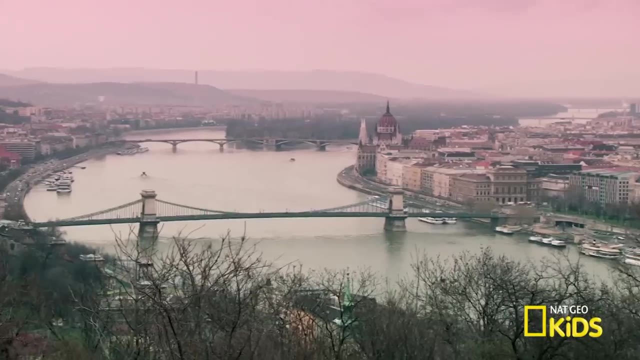 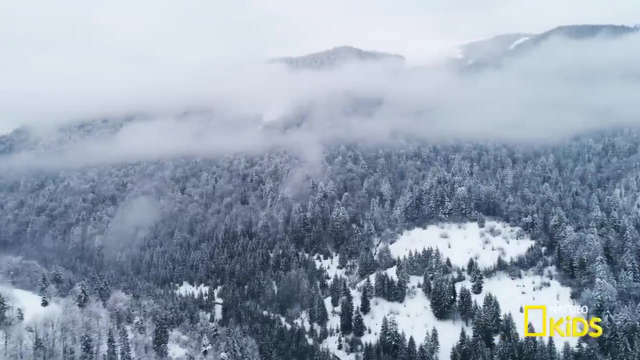 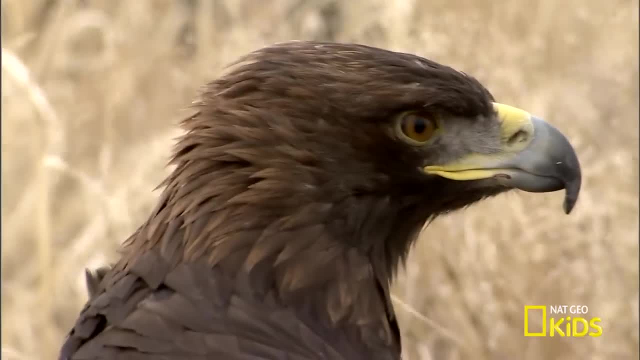 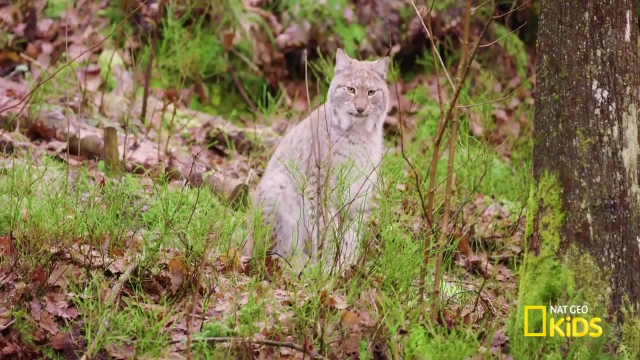 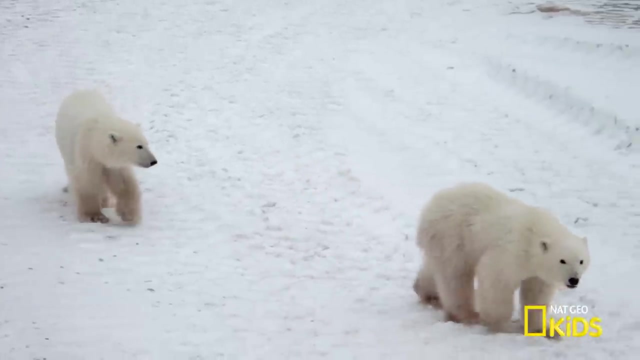 However at length. you may hear gray wolves howling, brown bears hunting or Golden Eagles soaring overhead In Eastern Europe. you may the see the rare Eurasian lynx and the European bison. On the Northern edges of Europe you may even see a polar bear Europe. 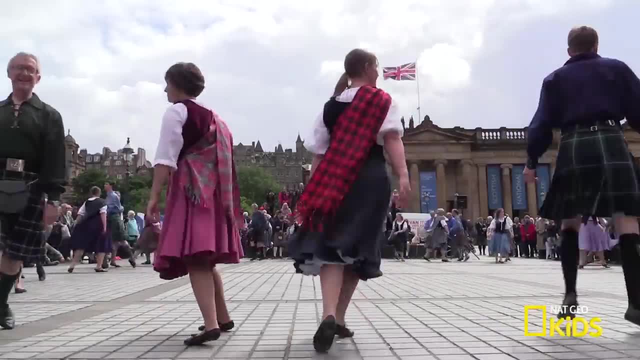 is packed with over 742 million people in 47 countries enjoying beautiful views, comforts and amazing plays ausge panora en avec bombs politiques et questions comm MBA ouvertes sur le context des maxima Nosferes aux États-Unis et des compétences de la qual.